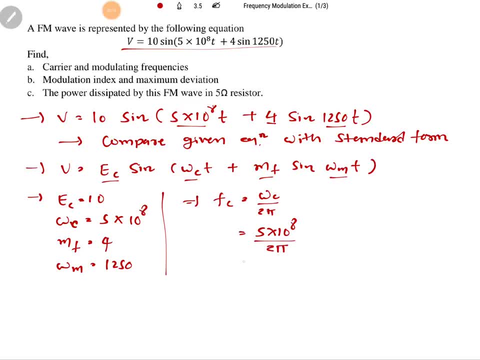 8 divided by 2 pi. So if you calculate these values, you will be getting 79.57 megahertz. Now, next is carrier signals frequency. So carrier signals frequency, that is what we have calculated, and then after we can calculate modulation frequency from this calculation. 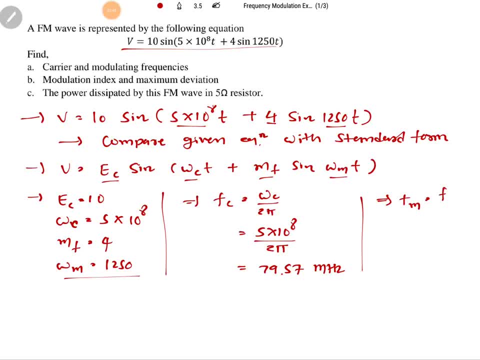 So f m, that is omega m divided by 2 pi. So omega m divided by f by 2 is effectiveness, that is 1250 divided by 2 pi. so from that we can have FM, that is 199 Hertz. now modulation index, now modulation index. that is what we have calculated M. 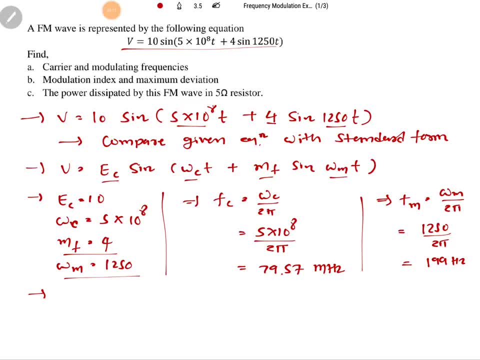 F is equals to 4. by comparing above equation with standard form. now from that we can say M F is equals to Delta F by FM. so we can have Delta F maximum deviation, that is M F into FM. now this modulation index, that is 4 and FM that. 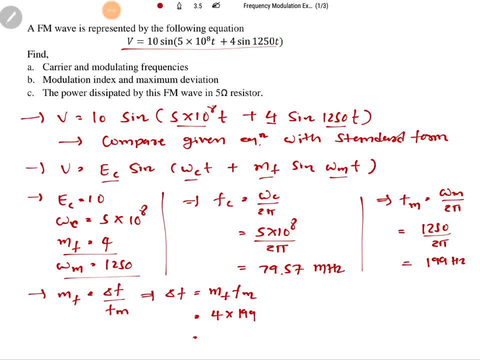 we have calculated 199, so this will result into 796 Hertz. and last parameter, now that we will be calculating, that is power dissipated by FM through 5 ohm resistor. so dissipated power, that is EC square by 2 R. now, if we 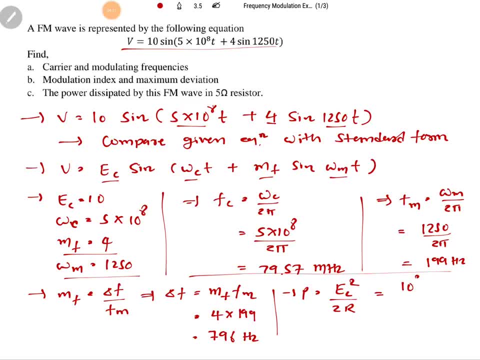 place values and EC is 10. so 10 square divided by 2 into R, that is 5. so this will result into power of FM signal, that is 10 volt, 100 divided by 10, so that will be 10 volt. so that is how we. 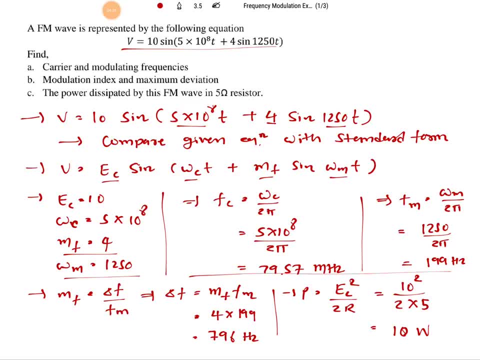 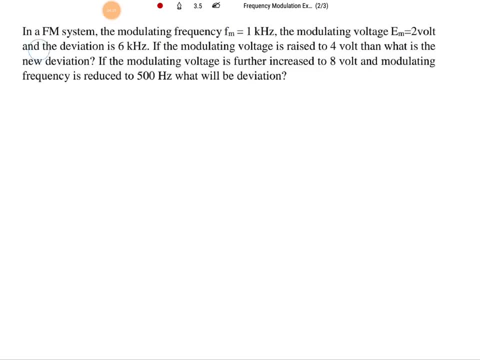 can solve this problem now. let us move on to next problem. now see, in this question, in FM system the modulation frequency, that is FM, is equals to 1 kilohertz. so let us mention all those things step by step. FM is equals to 1 kilohertz. so let us mention all those things step by step. FM is equals to 1. 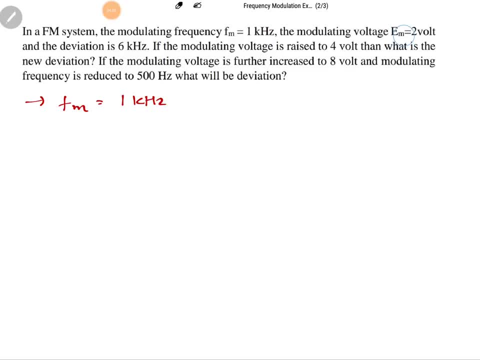 kilohertz, the modulation modulating voltage EM is equals to 2 voltage. so EM that is equals to 2 voltage and deviation is 6 kilohertz. so deviation that is 6 kilohertz if the modulation modulating voltage raise to 4 voltage. 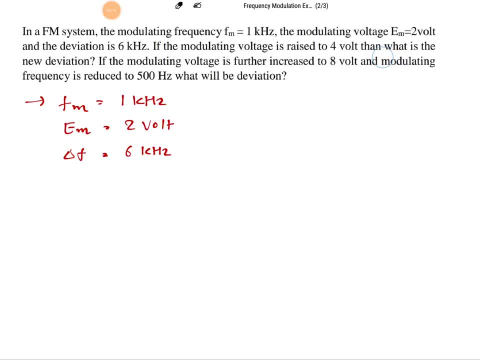 what is the new deviation? so if we change modulating voltage to 4 voltage, what will be new deviation? that is the question now here. first of all, this parameters are given to us and based on that we can utilize Delta F. and if you see my initial sessions, so where I have 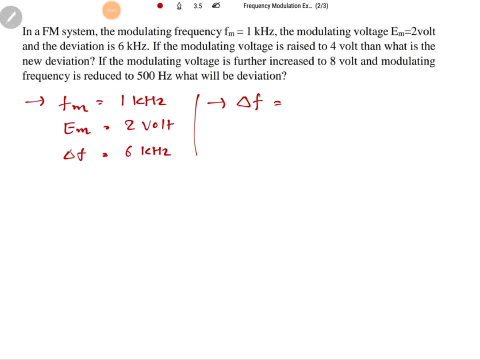 explained all those things. so Delta F, maximum deviation, that is frequency sensitivity into EM, and from this this we can calculate frequency sensitivity. so frequency sensitivity kf, that is delta f divided by em. now delta f, for initial case, that is 6 kilohertz divided by em, that is: 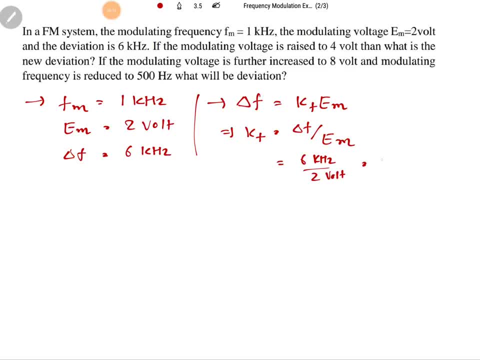 2 voltage. so we can say this is 3 kilohertz per volt. so frequency sensitivity, that is 3 kilohertz per volt. now if modulating voltage is raised to 4 voltage, then what will be new deviation? so now, if modulating voltage is raised to 4 volt, then what will be new deviation? so now, if modulating 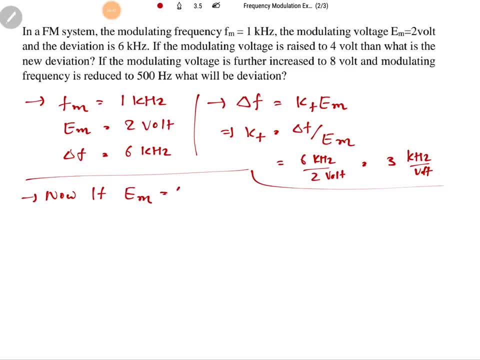 signal is having voltage that is 4 voltage. so new deviation, delta f, that we can easily calculate as per this formula kf into em. now kf that we have recently calculated 3 kilo hertz per voltage into em. that is 4 voltage. so new deviation that will be 12 kilo hertz. 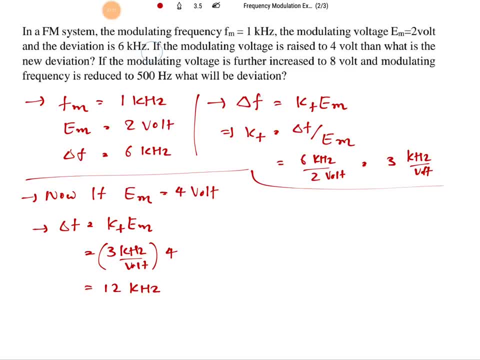 and then after it is, there is equation like: see, if modulating voltage is further increased to 8 voltage and modulating frequency is reduced to 500 hertz, then what will be new deviation? so here third case is there where now if em, that is 8 voltage, and fm, that is 500 hertz, then what will be new deviation? so we can calculate. 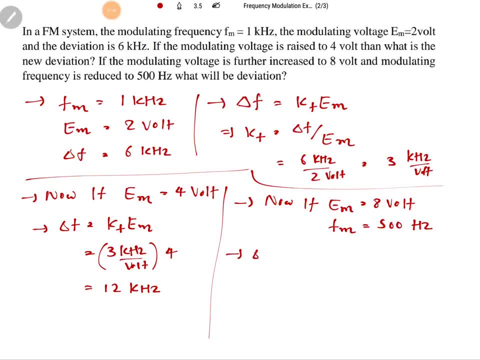 that as per delta f, that is 5.. KF, EM, where KF that we have initially calculated, which is constant, that is 3 kHz per volt, into new voltage, that is 8. so in that case, if we place these values so volt, volt will cancel. 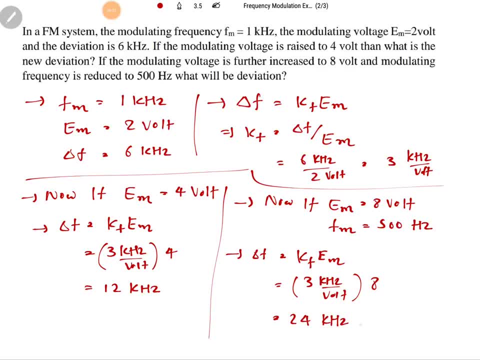 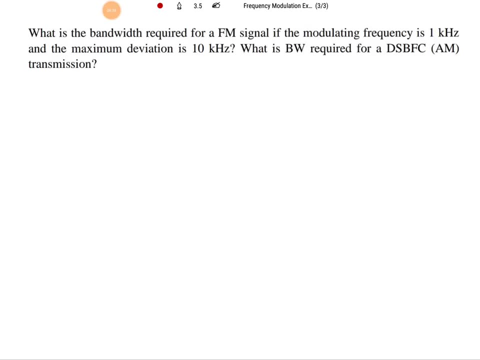 and then this will be 24 kHz. so that is how we can solve this problem. I hope that you are getting it and if you have any query, you just place that in command. let us solve next example now here in this question: what is the bandwidth required for FM signal if? 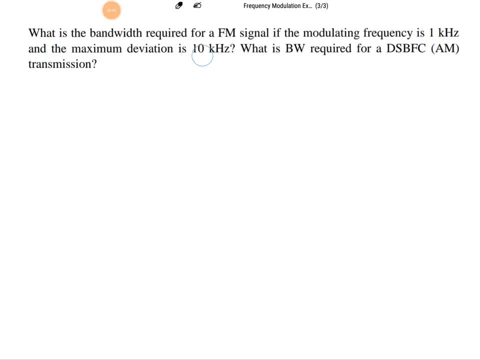 modulating frequency is 1 kHz and maximum deviation is 10 kHz. so here it is given for FM signal modulating frequency: FM that is 1 kHz, 1.5 kHz, kilohertz and maximum deviation that is 10 kilohertz. so as per Carson's rules, 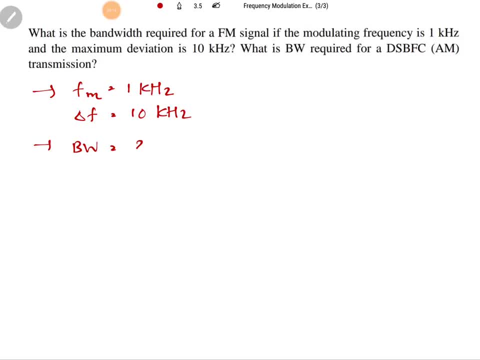 bandwidth that we can calculate and that is 2 into FM plus Delta F, so FM that is 1 kilohertz, Delta F that is 10 kilohertz, so this will be 22 kilohertz. now here in this question, what is the bandwidth for DSB FC AM transmission? so if you see,